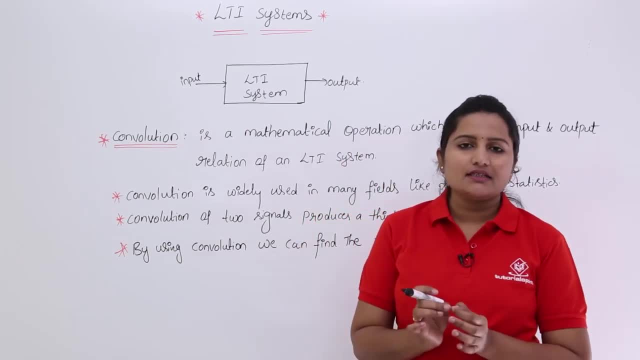 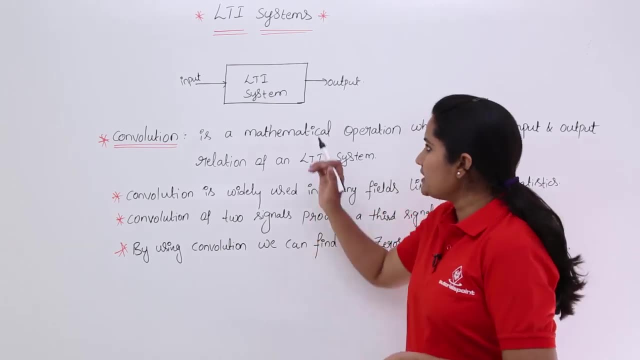 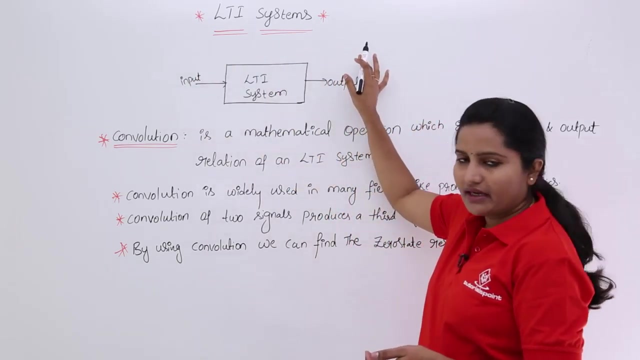 particular LTI system. That means if you want to consider the system, impulse, response and input relation, to get output you need convolution. That means, for example, if you are having any LTI system, you are having any example or input and you are having any output or response. So here I am considering that output. 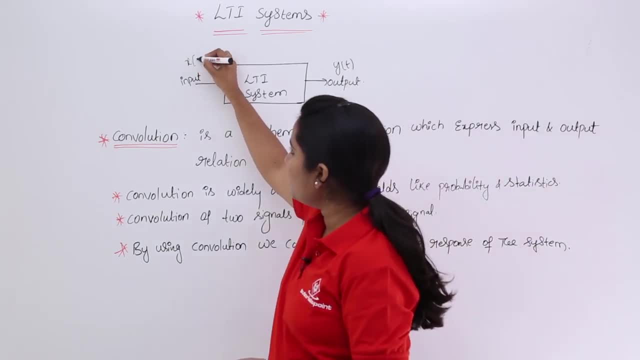 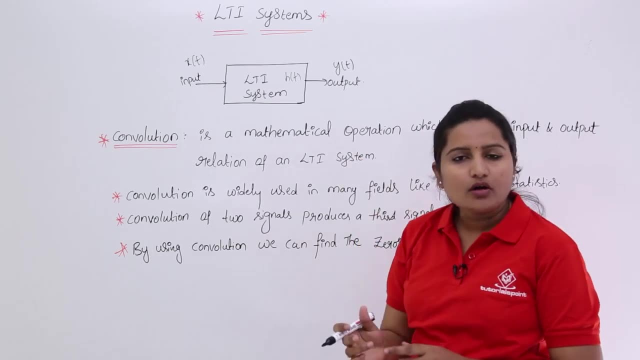 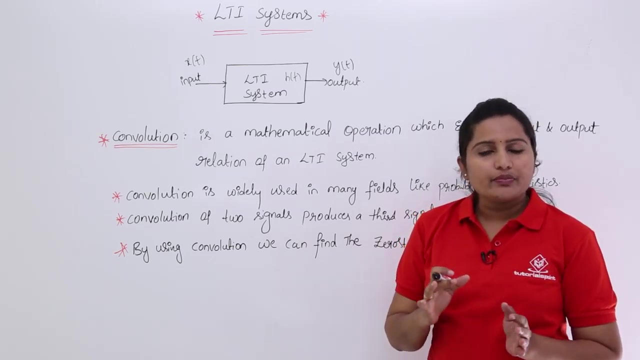 or response as y of t and input as x of t, and your system, LTI system, is having some impulse response- h of t- Then if you want a relation between output and input and impulse response of the system, then you require convolution. So before getting into the equations for 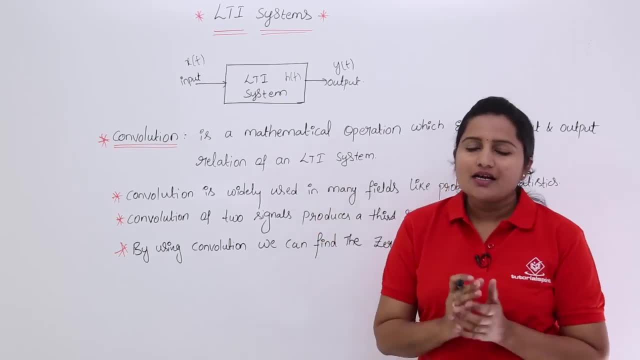 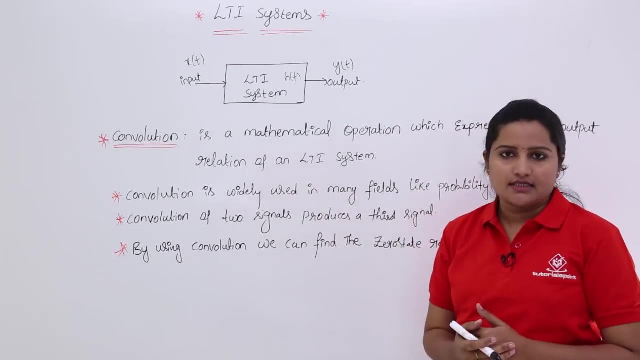 output. So we are going to discuss about convolution here. Convolution is nothing but a mathematical operation which express input output relation of a LTI system. Convolution is nothing but a mathematical equation or operation. So which is going to provide the 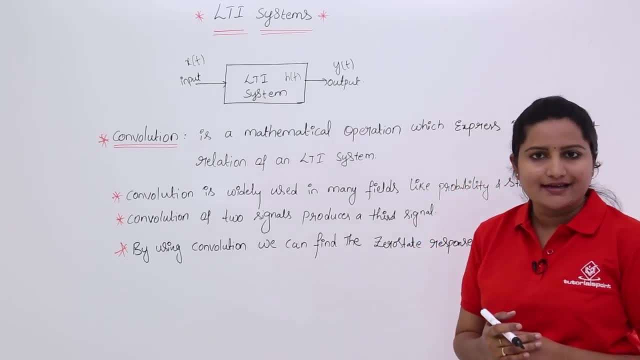 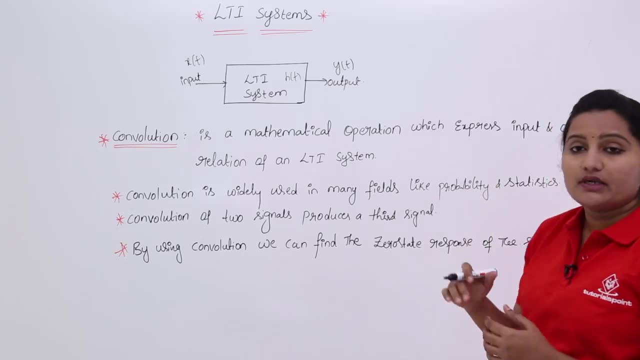 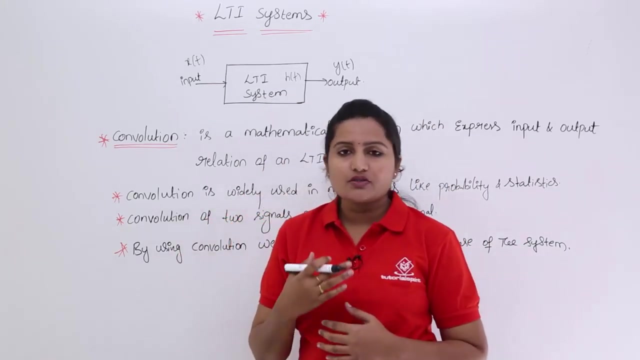 relation of input, output and impulse response of a LTI system. Coming to convolution, convolution is widely used in many sectors and many fields like probability and statistics. and here, convolution is widely used in many sectors and many fields like probability and statistics, Convolution of two signals always produces a third signal That means it is going to 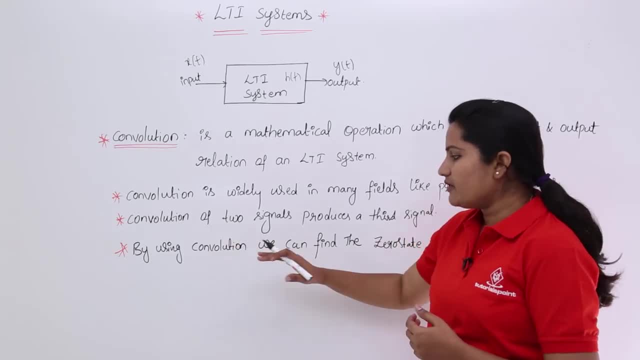 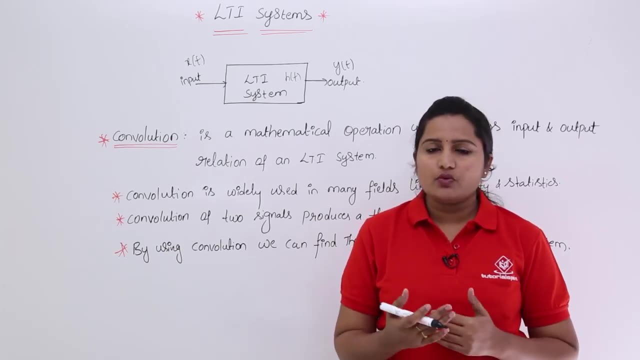 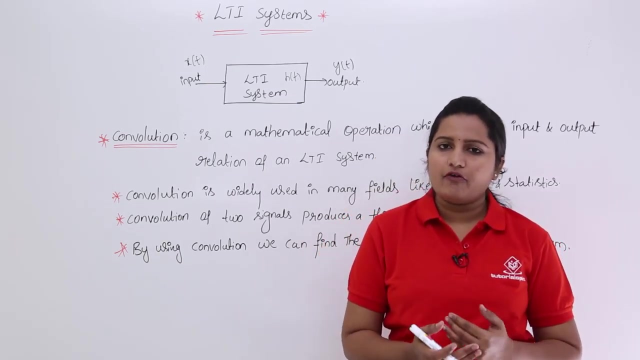 produce a different signals. So here, by using convolution, we can find the zero state response of a system. So many times in any technical exam they will ask: what is the zero state response of the system? Then that zero state response of a system can be found by using 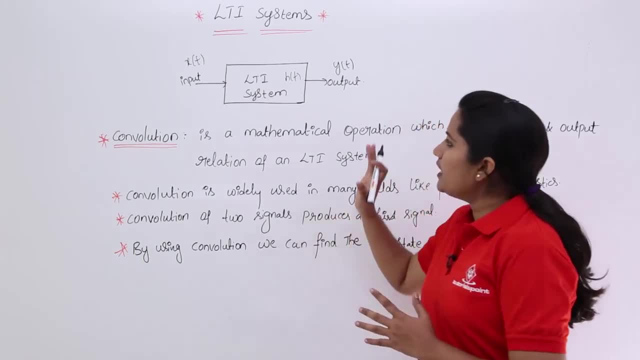 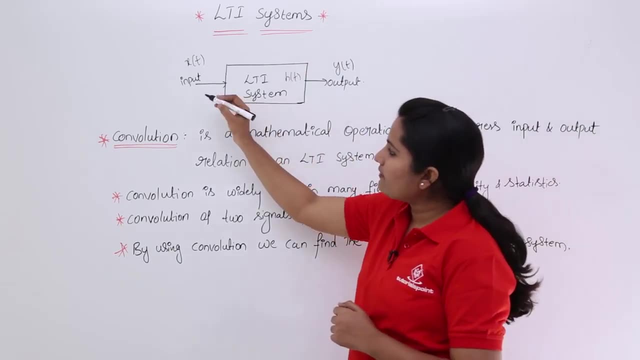 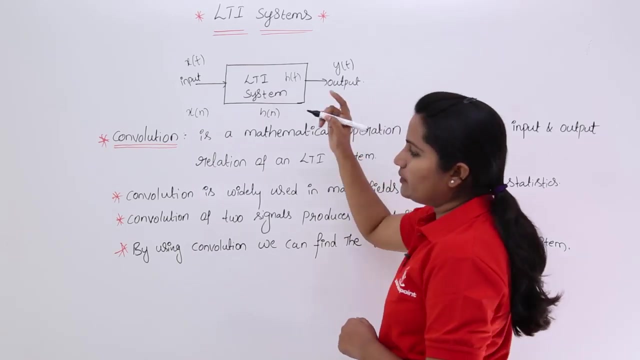 convolution of the system. So here, if you saw, this is continuous system, continuous convolution. So whenever you are having x of n, So x of n and h of n and y of n as your input of system and impulse response of the system and output of system, 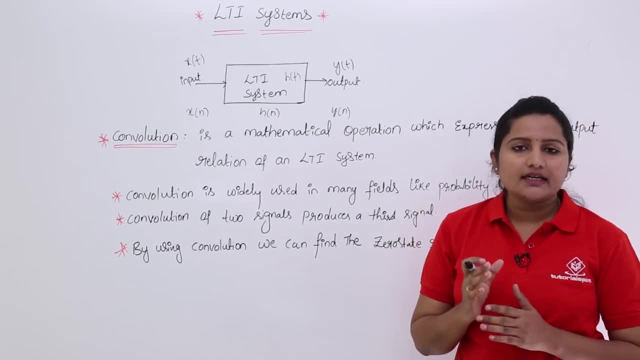 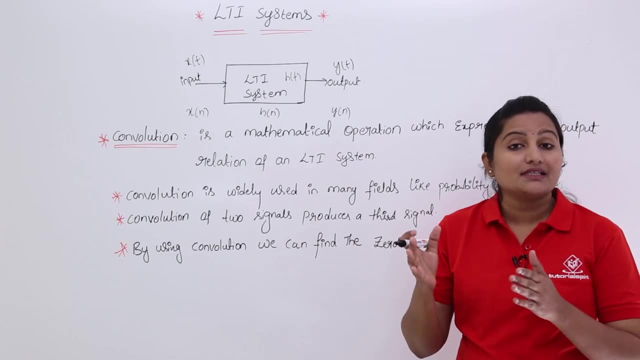 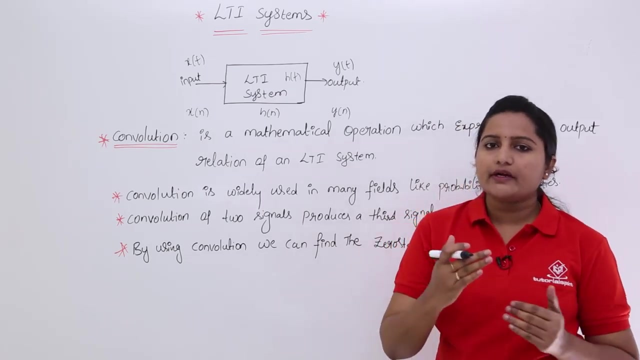 that convolution is called as So discrete convolution. that means if you want the relation of your system output, input and your impulse response in discrete domain, then you need to consider your discrete convolution. So you need to consider your discrete convolution. If you need your output, input and impulse response relation in continuous domain, then 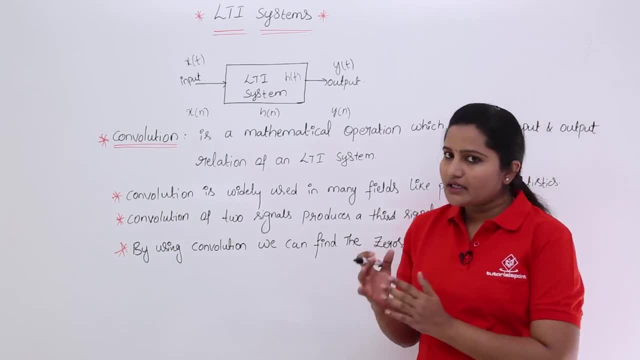 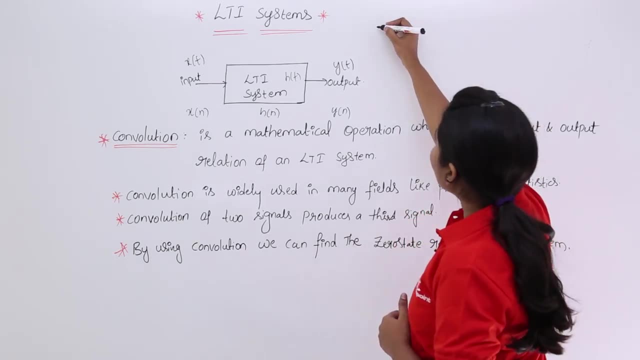 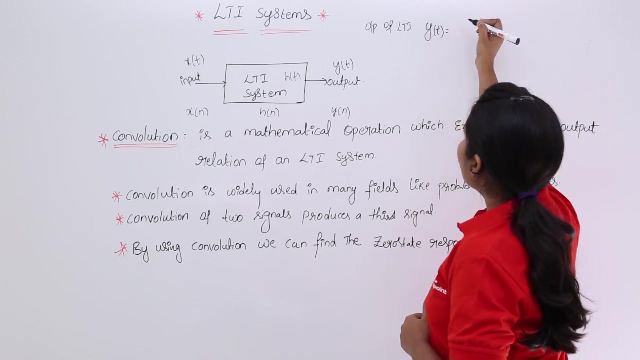 you need to use your continuous convolution. Now I will give you the equations for continuous convolution and discrete convolution. Now here the output of LTI. output of LTI can be noted as: y of t is equivalent to x of t. convolution with h of t. Like this we can represent the: 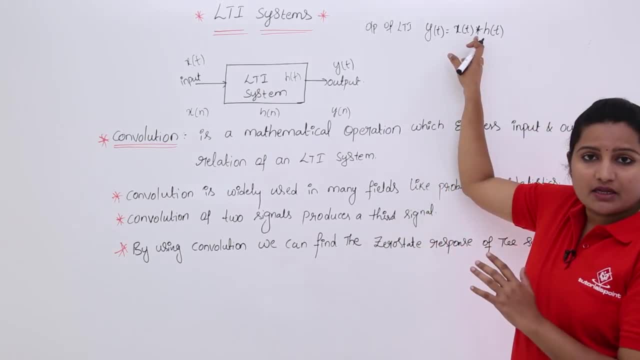 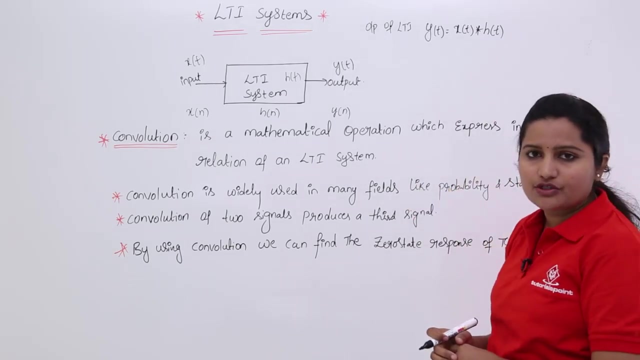 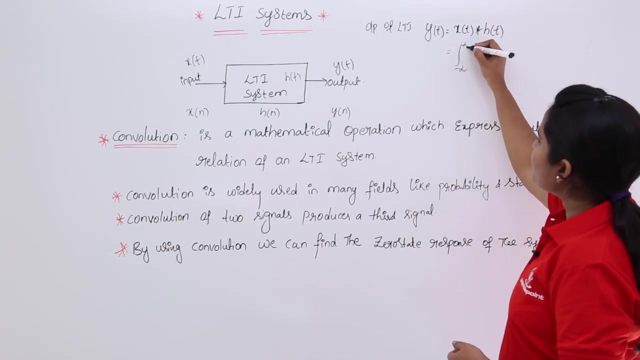 convolution. This is the symbol for convolution, star is the symbol for convolution, and here always the LTI system. output is equivalent to input, convolution with impulse response. Then what is the meaning of this star, what is the meaning of this convolution? If you written x of t, star, h of t, then this is equivalent to integral minus infinity to infinity. So 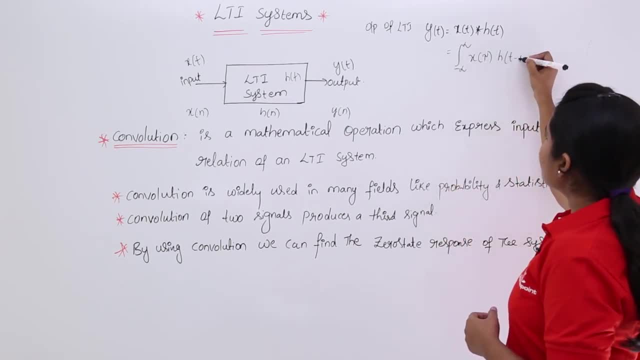 x of tau, h of t minus tau, y of t minus t, Hence y of t will be equal to h of t minus tau, h of t minus tau, plus tau, t will be equal, And if, which she describes it is that this will be equal to inralkommen tape, but approximately this is infinite. so expression is 1, what is the? 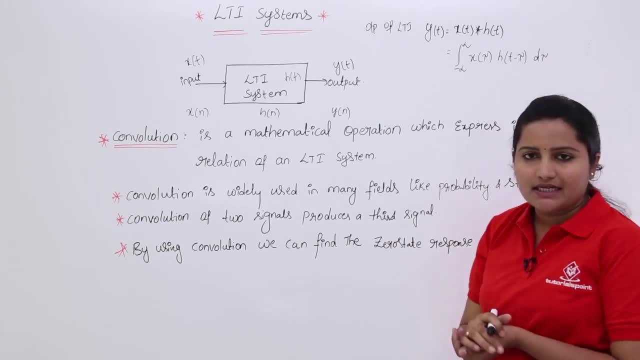 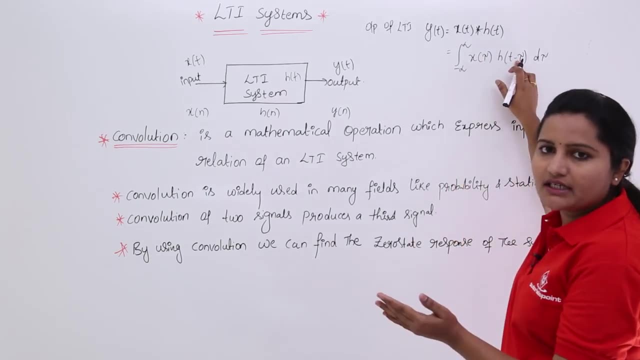 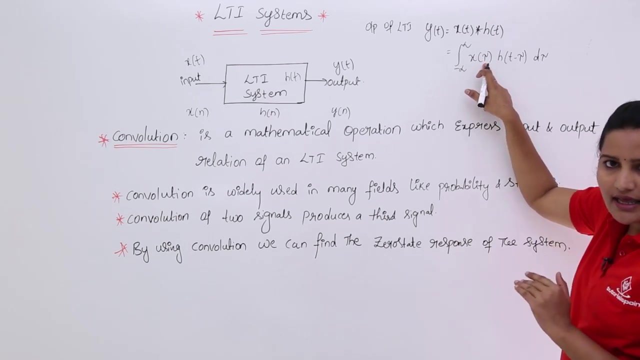 d tau. so here, by observing this equation itself, we can say convolution is nothing but sliding one signal over reflected and folded and shifted signal. this is actually, for example, this t, if i consider like mine tau. so if i consider like mine tau here, if minus tau, if you are having in. 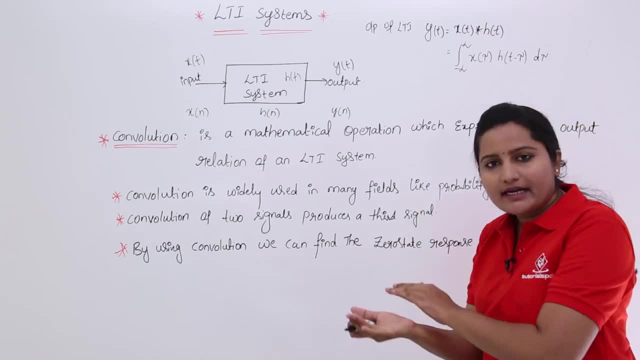 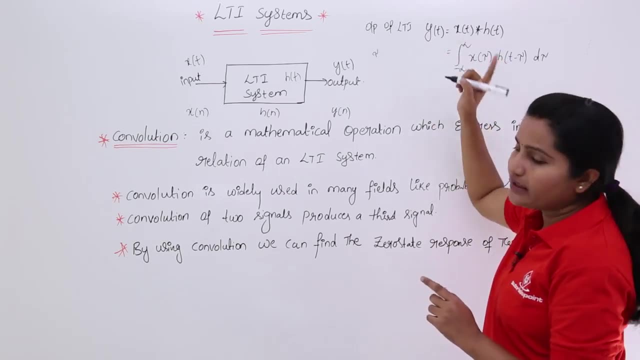 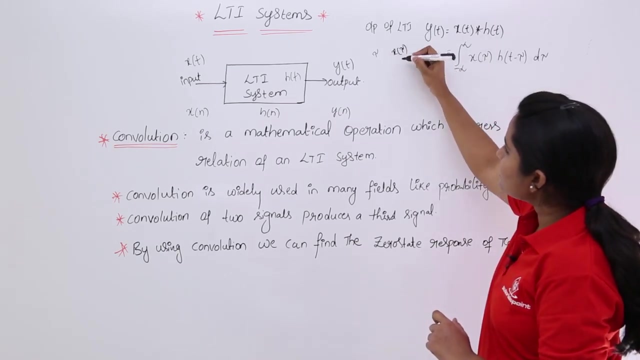 impulse response. that means that is a folded signal, actually shifted means. so, for example here, so tau, i am considering, like my time period, present time period, and here for the time period, my signal x of t slides over this signal. this signal is a shifted impulse signal. that means 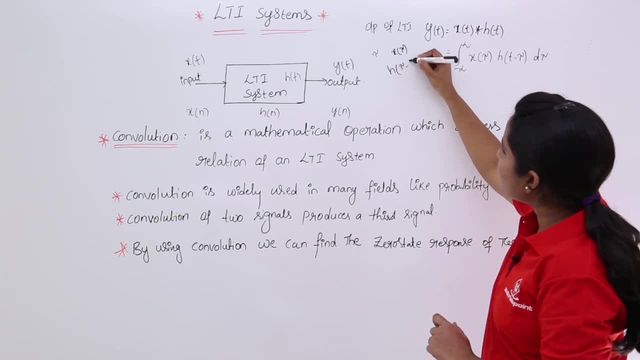 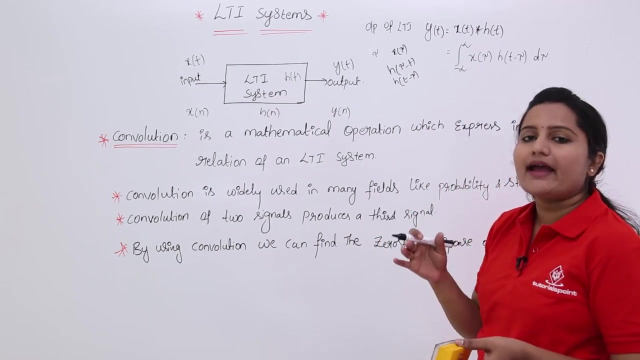 so h of tau minus t will be its shifted impulse response and it will become folded signal when you are giving so t minus tau, so when you are giving reversal, time reversal, then that is called a folded and shifted signal. so by observing this equation itself we can say: 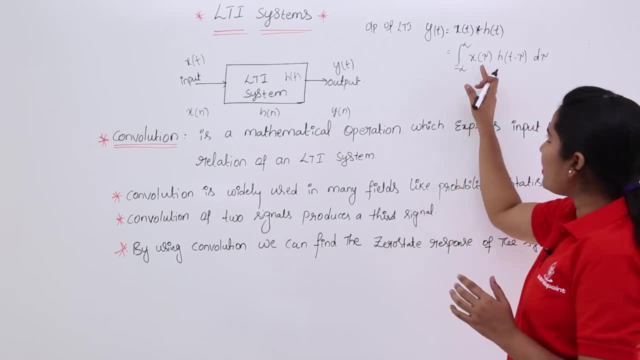 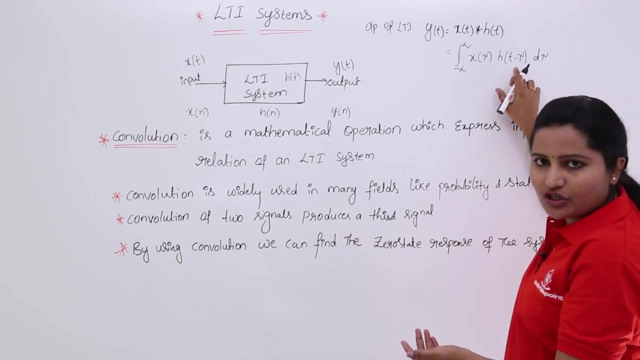 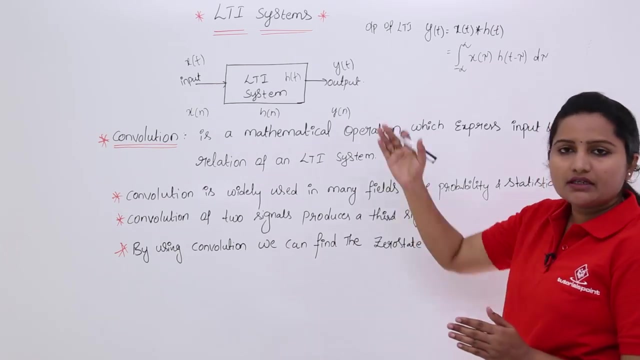 convolution is the process of sliding one signal over folded and shifted version of other signal. so this is folded and shifted version of impulse response. and here is your input signal. so sliding of input signal over folded and shifted version of impulse response will provide you convolution of those two. so that is nothing but y of t. so here, in the same way, you can write this same equation. 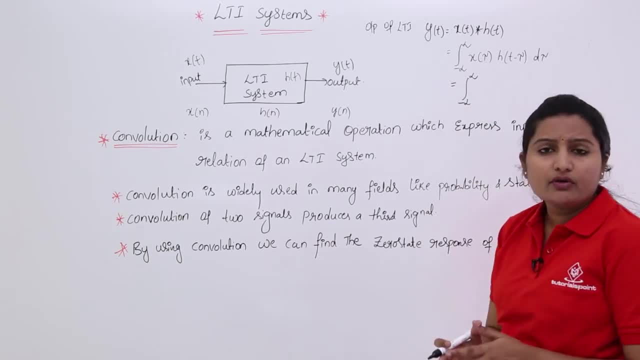 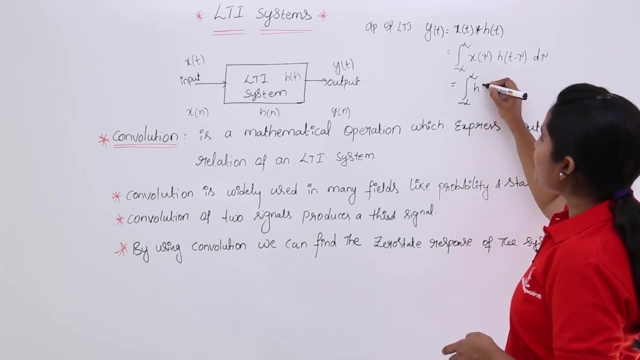 so that means you can keep your impulse response as it is and you can fold and shift your signal. x of t, that means like this also: you can write so: h of tau, x of t minus tau, d tau. also you can write as x of t, convolution with h of t, like this or like this: you can do, you are going to get. 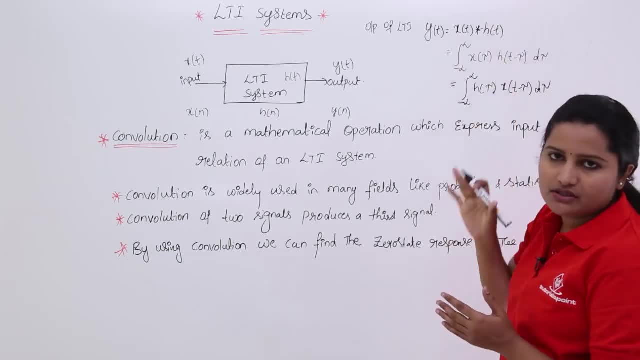 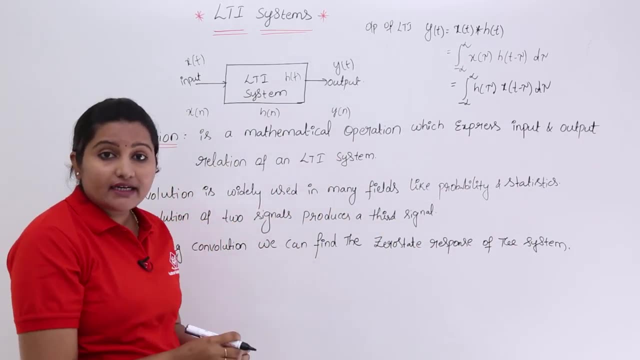 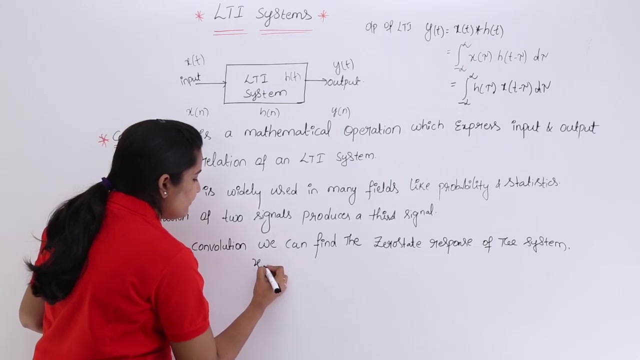 same thing. so that means this is about continuous convolution. coming to discrete convolution, if you are going with discrete convolution, that means you need discrete response of a system for a discrete input and discrete impulse response. then that x of n is equivalent to sorry. y of n is equivalent to output or response of a system. y of n is equivalent to x of n convolution with h of n. 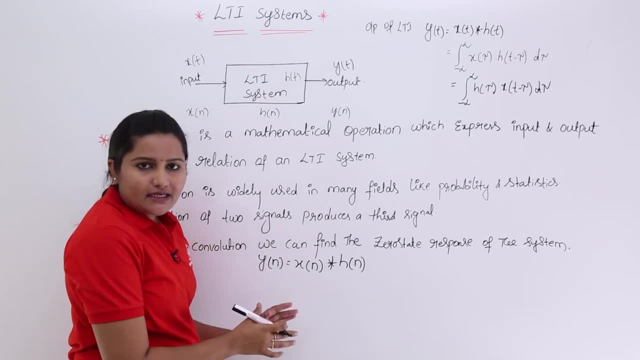 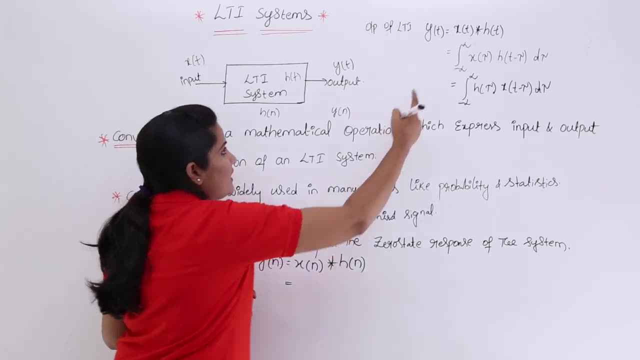 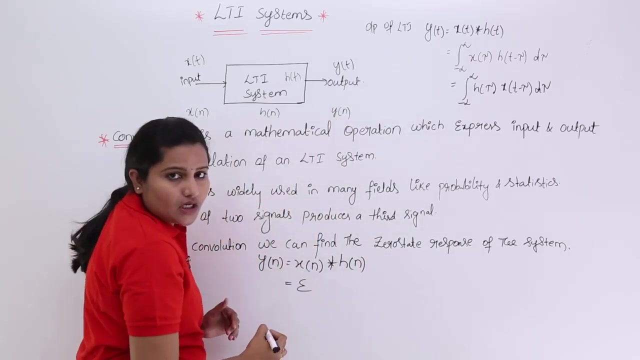 now similar to here I am going to represent with a equation for this term. that means: what is the discrete convolution equation here? whatever integration is there that I am going to convert into summation, as we are in discrete mode. so summation k is equivalent to minus infinity, to. 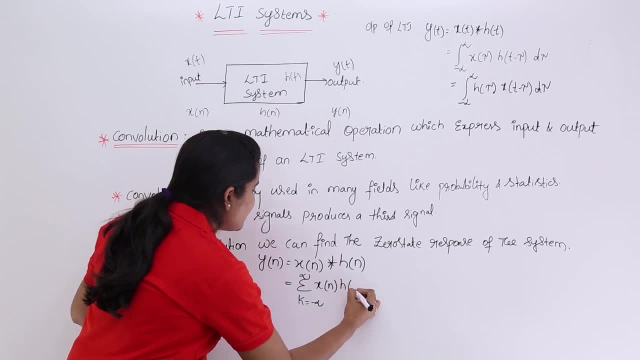 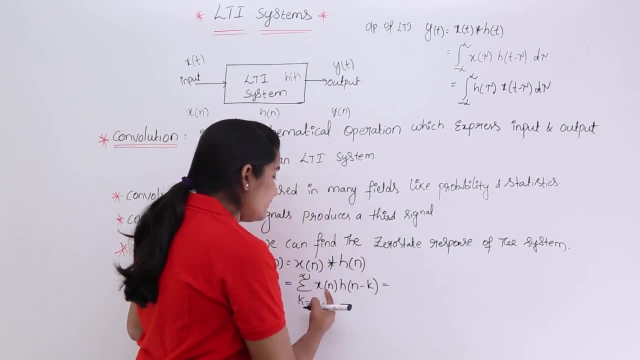 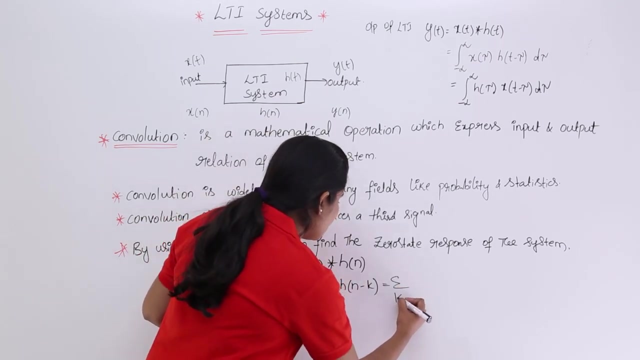 So x of n, h of n minus k is the discrete convolution value. So similarly we can shift x of n and we can put it as it is, as h of n. So that means we can write like this also: k is equivalent to minus infinity, to infinity, h of n, x of n minus k. So like this also we can write 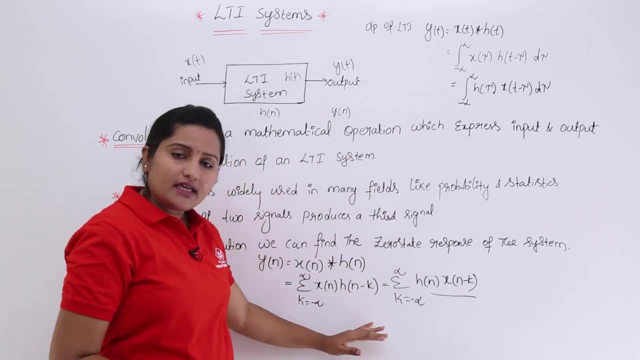 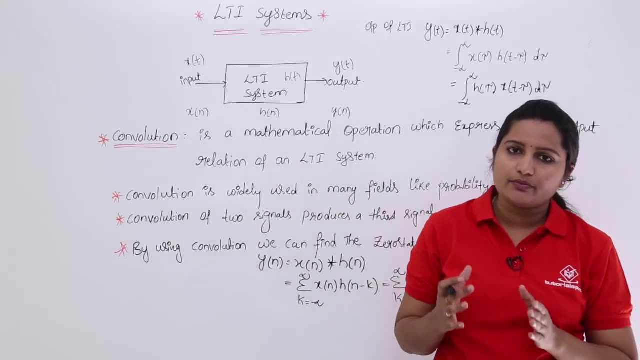 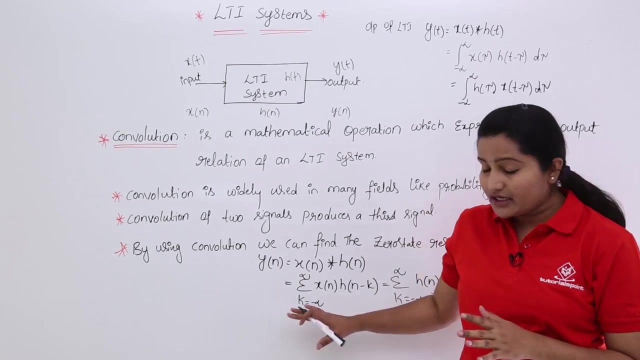 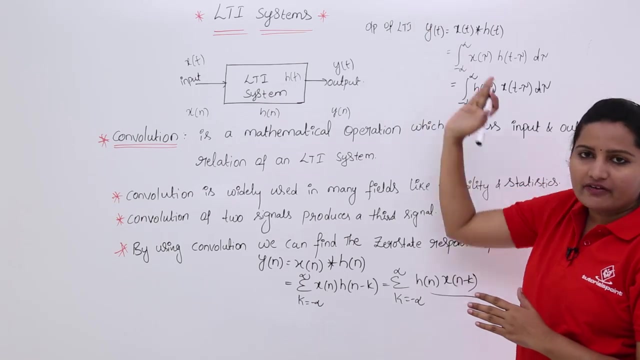 So this is continuous convolution here. this is discrete convolution. Mostly we are going to use continuous convolution in problems. Definitely you are going to get problems on continuous convolution. 90 percent of the problems will come from continuous convolution, but discrete convolution also very important. So here, whatever we are having as output of LTA, 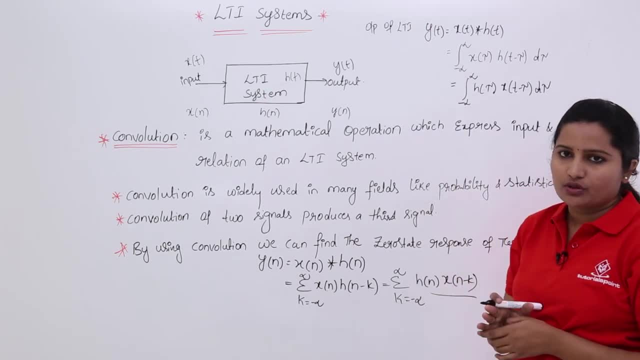 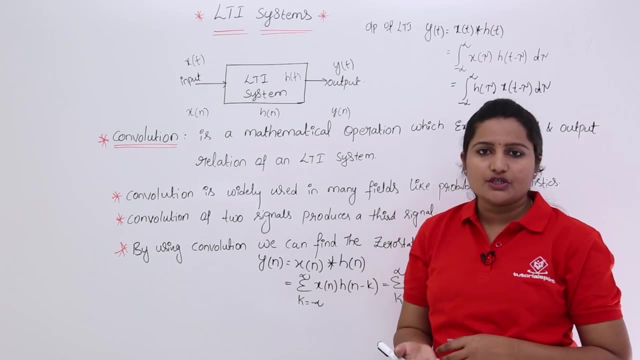 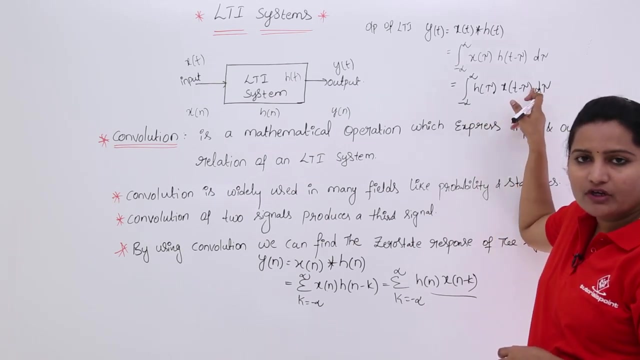 system that can be described by convolution only. The equation for convolution is always like this: Integral minus infinity to infinity, x of tau, h of t minus tau, d tau or integral minus infinity to infinity. just keep this impulse response as it is and fold and. 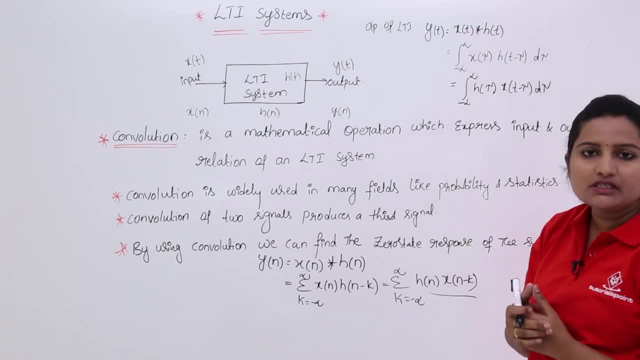 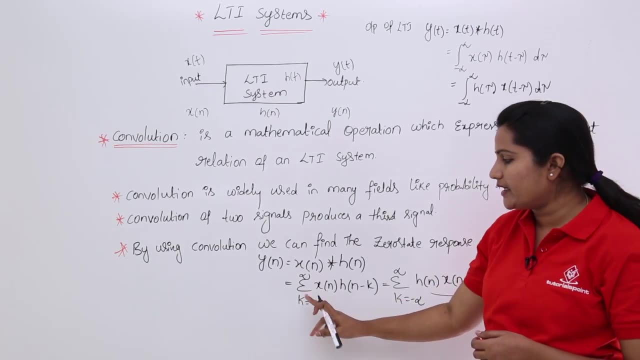 shift your signal, then you are going to get same continuous convolution formula. So here, in place of integration, if you substituted summation, then you will get a discrete formula and you need to replace that t with n. So y of n is equivalent to always, the discrete convolution is equivalent. 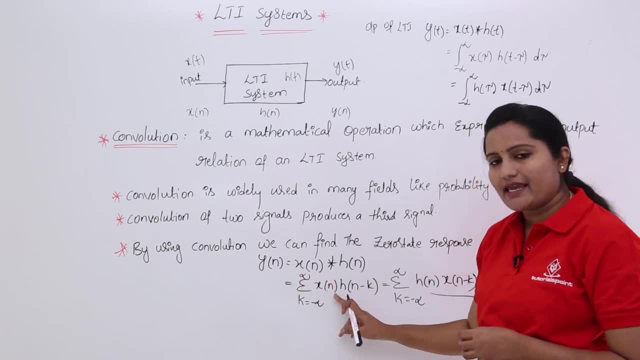 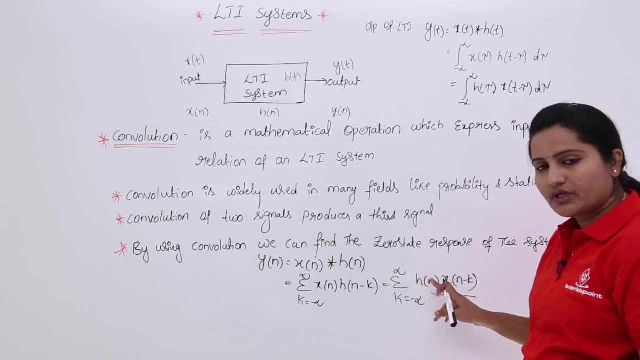 to n, So y of n is equivalent to always. the discrete convolution is equivalent to n, So y of n is equivalent to summation k, equivalent to minus infinity, to infinity x of n, h of n minus k. or you can use this formula: summation k is equivalent to minus infinity, to infinity h of n, x of n minus. 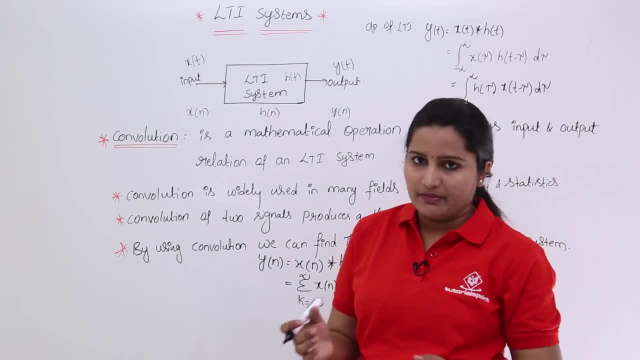 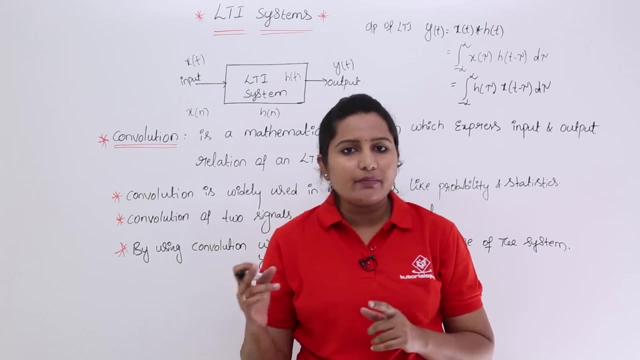 k Why I am discussing two-two formulas for each means. for example, you are given with any signal and impulse response, So shifting of signal is easy or impulse response is easy. you need to check So you can use according to that. That means, for example, you can use according to: 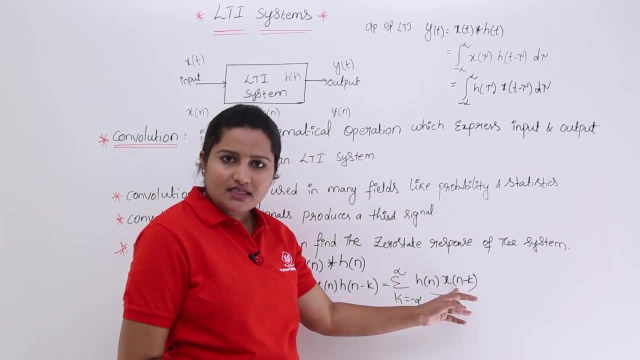 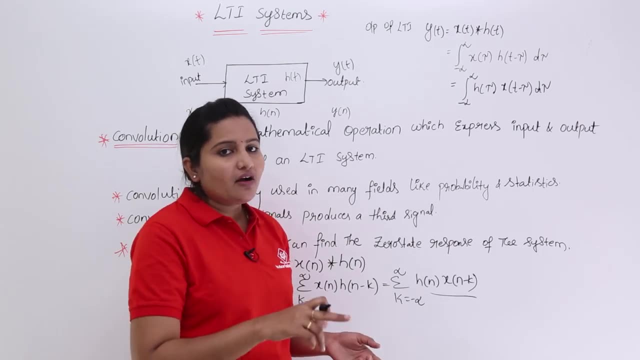 that, So you can use according to that. That means, for example, you can use according to any problem: shifting of x of n is easy and h of n is typical. then you are going to use this formula, For example, in any other problem. shifting of impulse response equation is easy. That means: 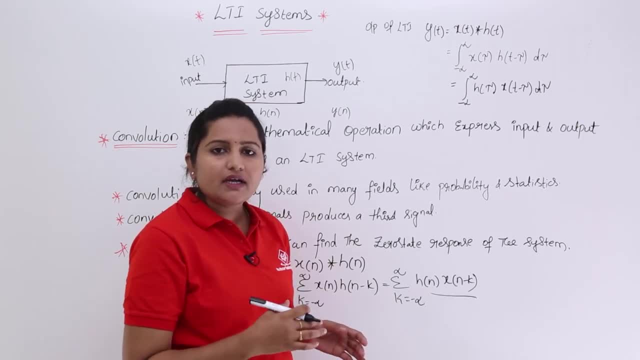 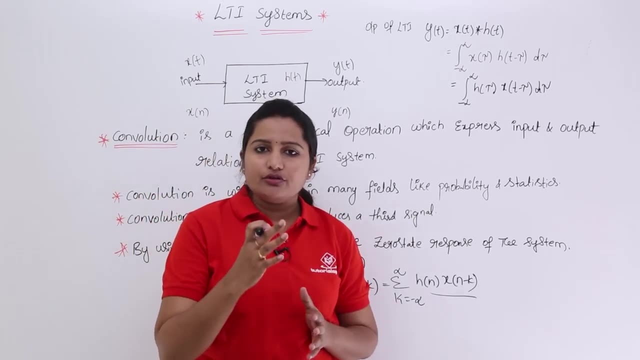 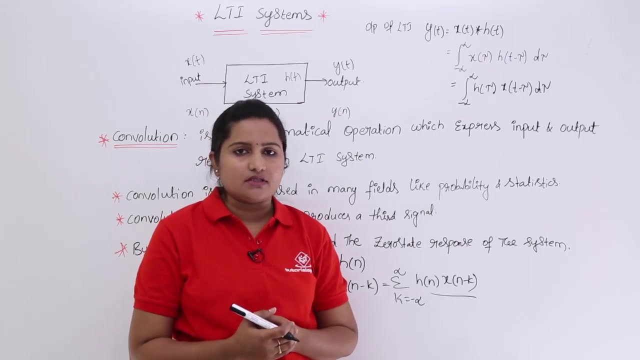 applying shifting for that equation is easy, but it is typical to apply shifting and folding property for signal. then you are going to choose this formula. So, according to your feasibility, you need to choose the formula that to calculate convolution of continuous or discrete time system.